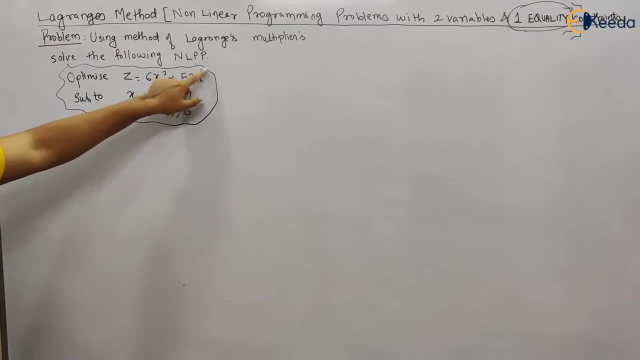 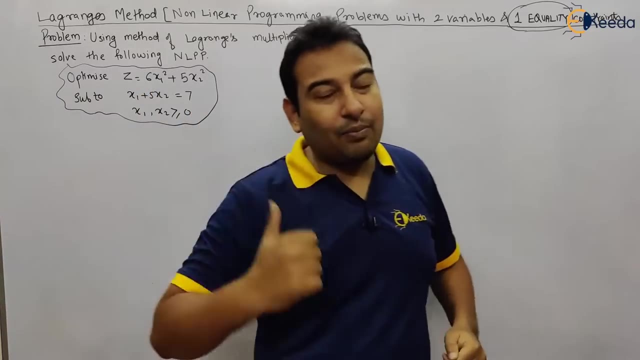 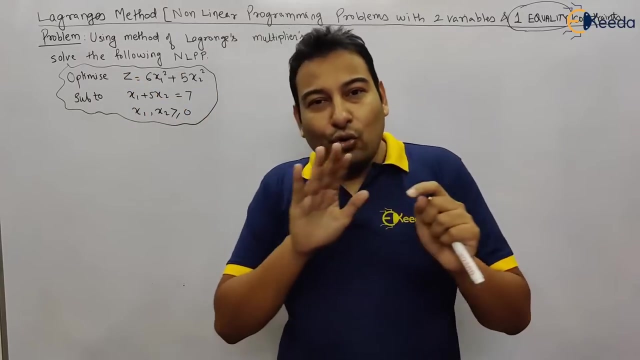 find relative maxima or minima. This is the function given and with this function we do have one constraint. So this is the difference between this type and the previous type. If you observe the previous type, there was only one objective function, There was no constraint, But in 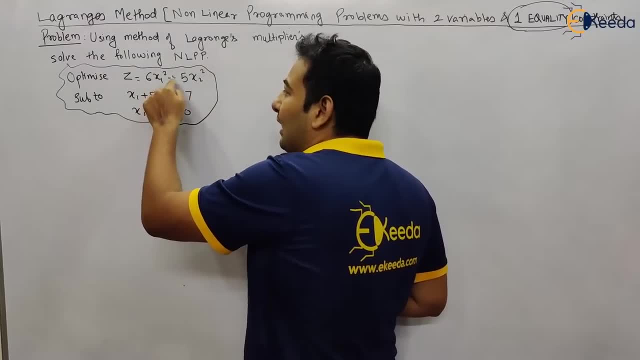 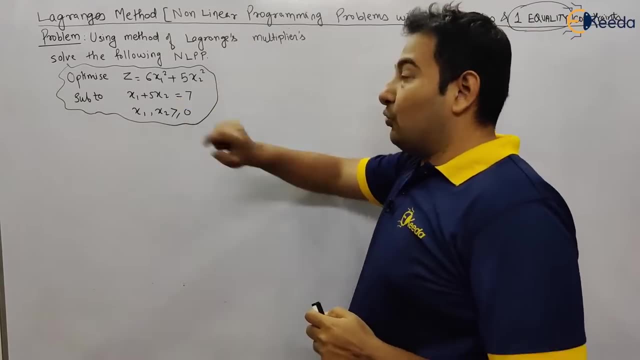 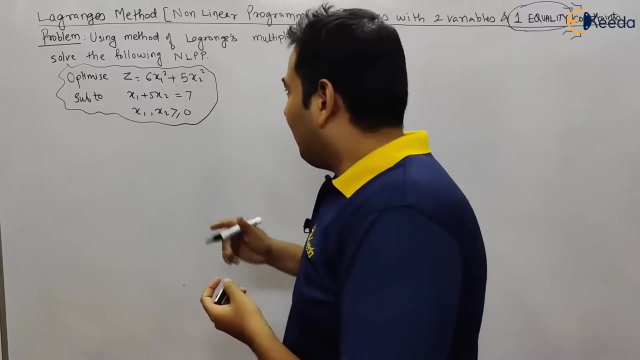 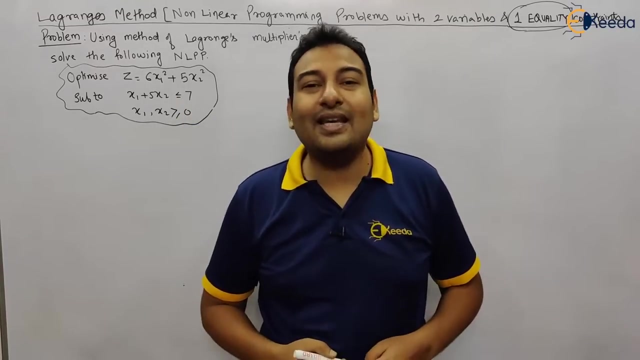 this particular problem, objective function is given. along with that, one constraint is given in the problem, and that is also equality constraint. See this: equal to This. equal to indicates equality constraint. Suppose the same problem, but here suppose it is less than equal to. then in that case this constraint will become inequality constraint, inequality. 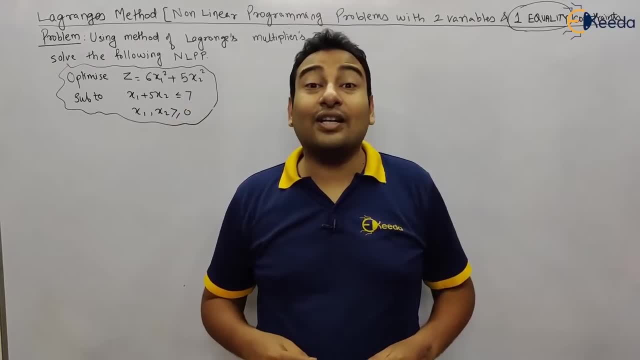 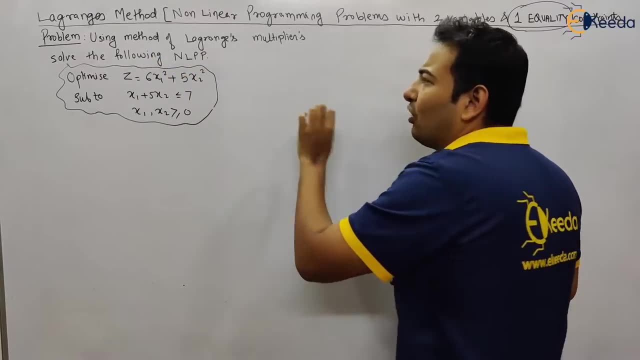 constraint and the problem will belong to the next type, that is, a contact car. so you should be very careful. see it's clearly mentioned in the problem. use Lagrange's method or Lagrange's multipliers to solve this equation. and here it is equal to. but what if it is not given in the 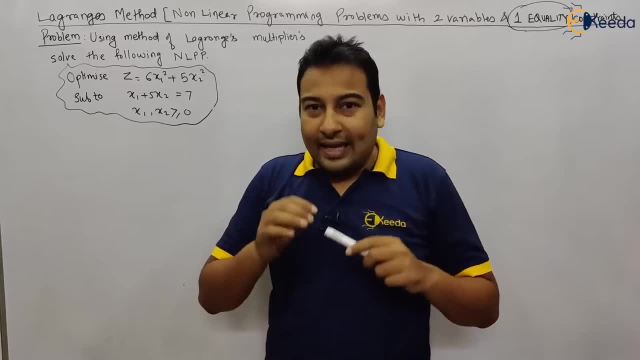 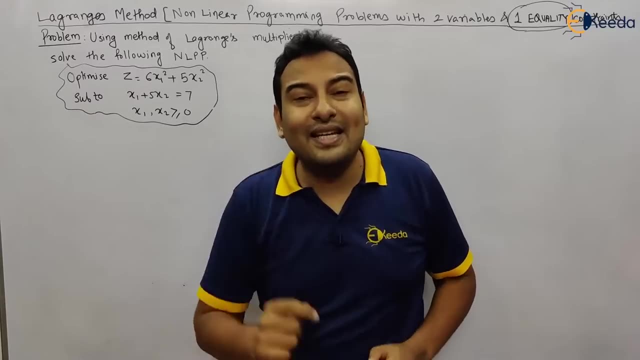 problem and it is asked to optimize it. in that case you need to identify: if it is equal to, then it is Lagrange's. if it is less than equal to, that means inequality. then the problem will belong to contact car. so you should be very careful about that. so let us start. so this is the problem given. 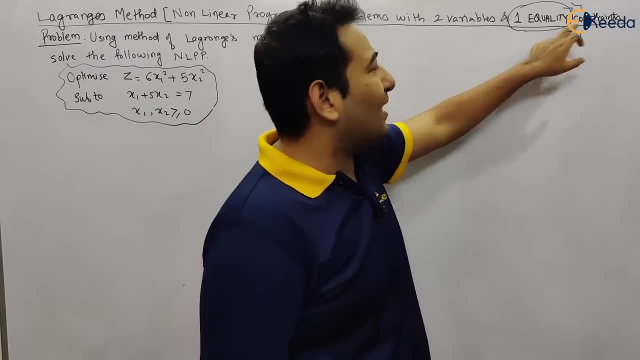 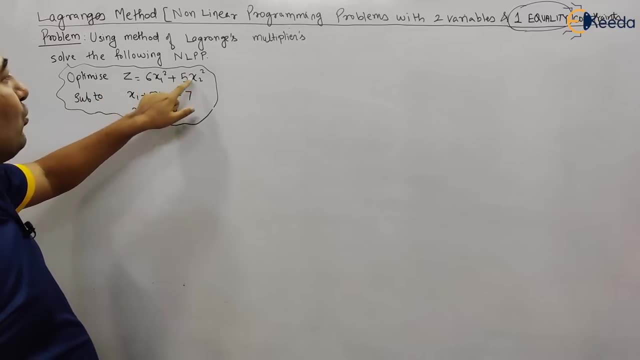 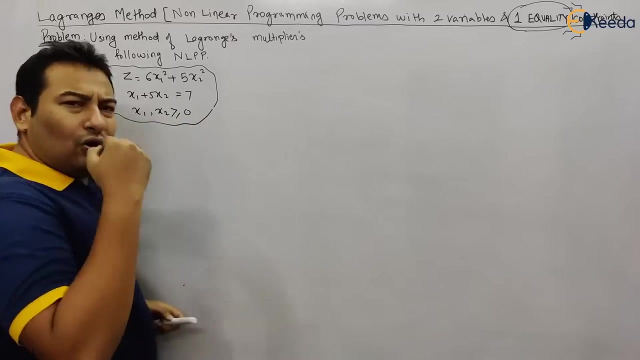 and it's two variables and one equality constraint. so it's clear: there is one constraint and equality constraint and there are only two variables, x1 and x2. and this is your last equation, and this is common for all the problems of N, LPP or LPP. LPP means 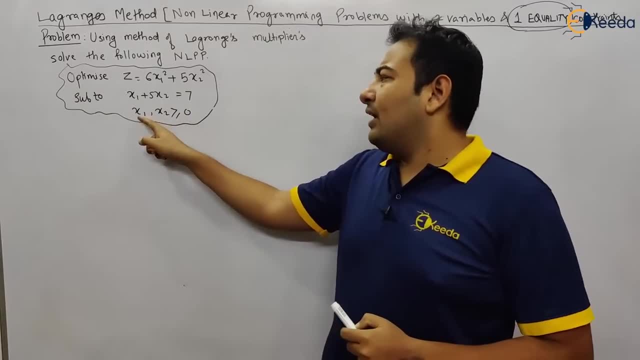 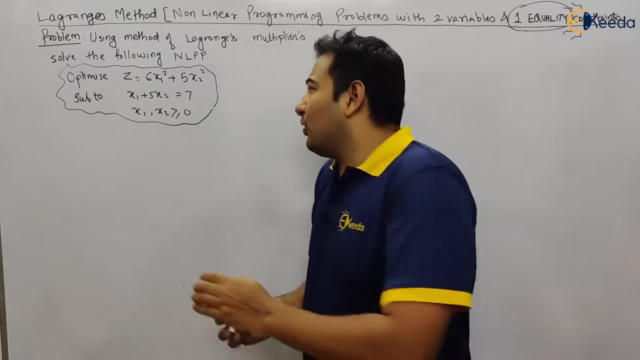 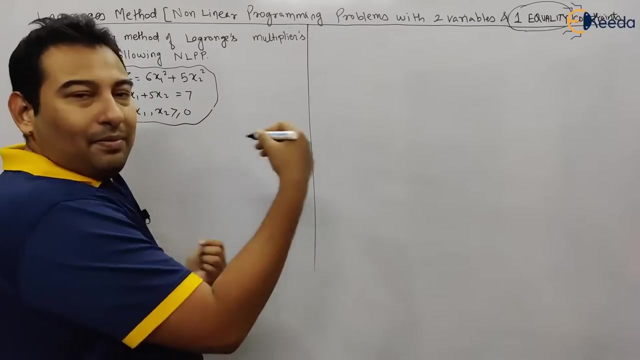 linear programming problem. this last line will always be given x1, x2 greater than equal to zero, so ignore it. so it doesn't. it's not useful for us in this particular type, so ignore this. basically, we're going to focus on this, okay, so let us start. remember the last type in which we discussed. 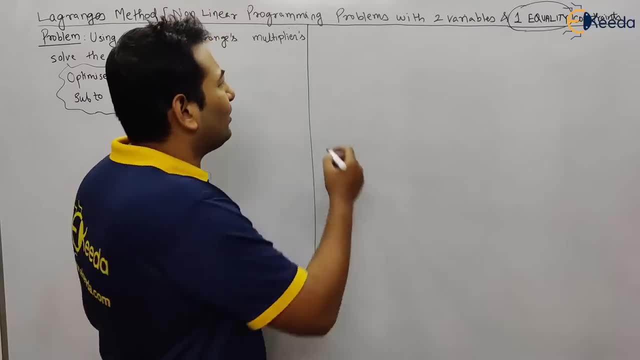 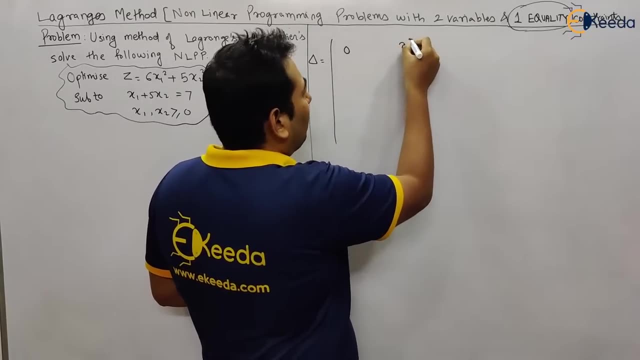 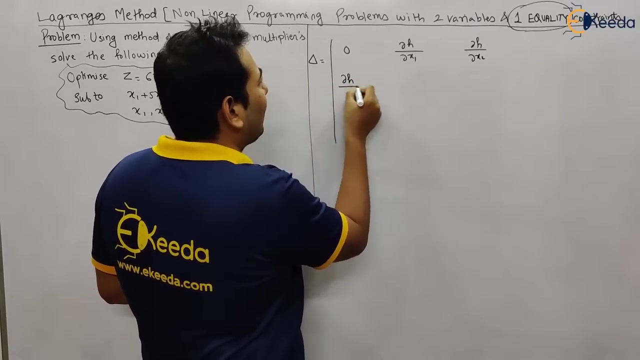 hashen matrix: here also there are few conditions. so let us check what are the conditions for maxima or minima? in that case, we're going to find out. Delta: here it will be zero: dou h upon dou x1, dou h upon dou x2. I'll explain you everything, so just wait. what exactly this x h? okay, now here we're going. 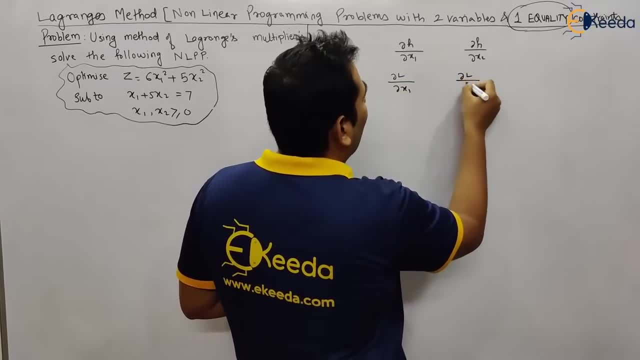 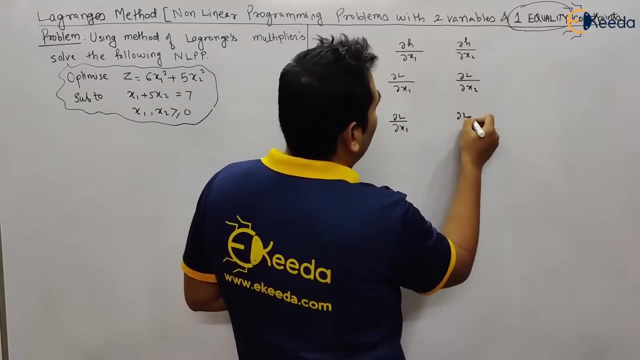 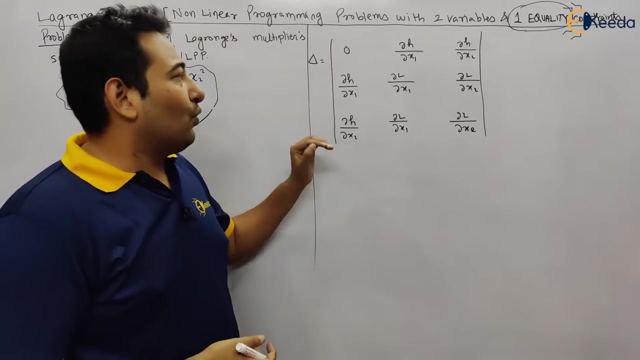 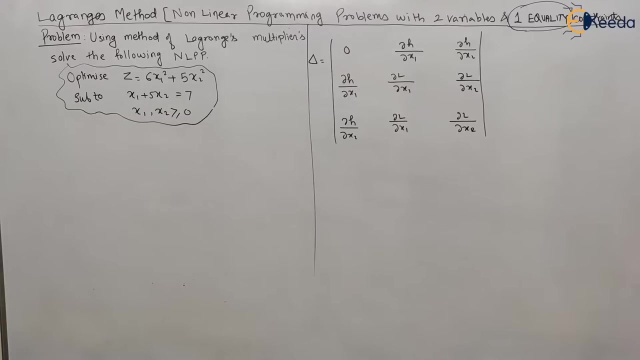 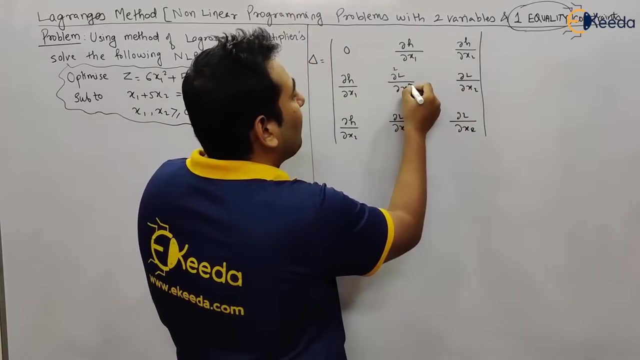 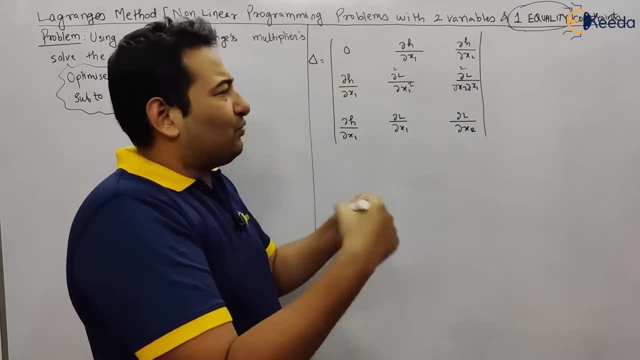 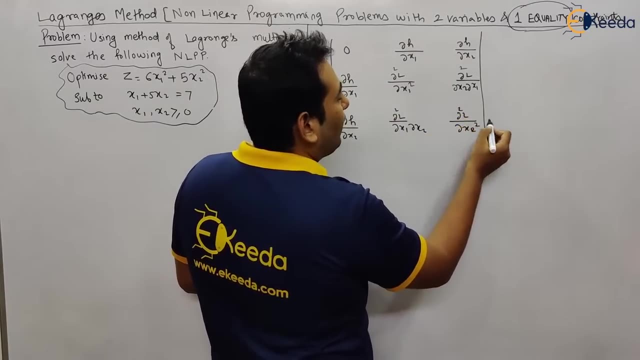 x2 and dou x1. so it doesn't matter if you write dou x1, x2 or x2- x1 doesn't matter- and if you're going to differentiate with respect to x2, so this will be x2 and x2 square. so this is your delta and this delta will determine. 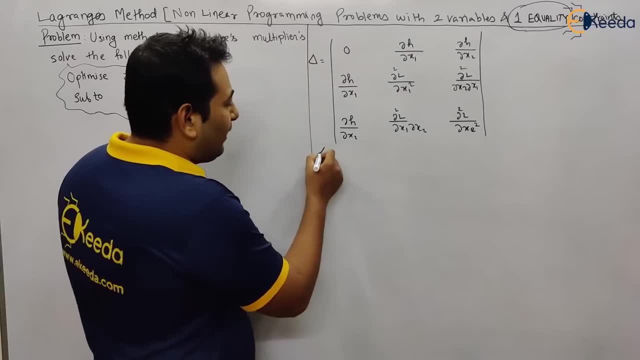 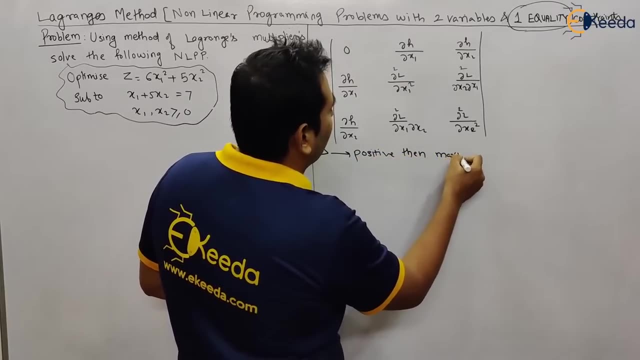 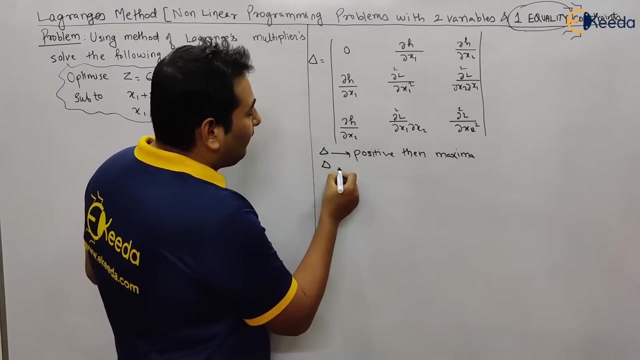 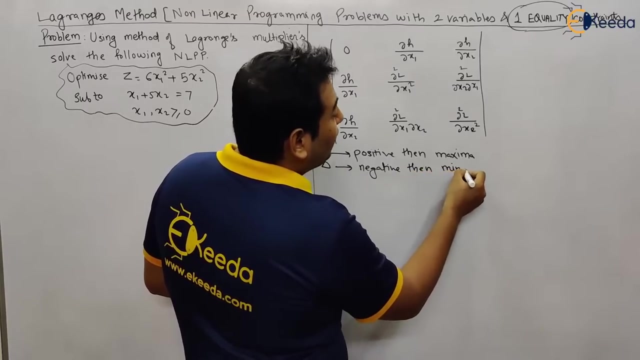 whether the answer is maxima or minima. if delta is a positive, then maxima. we're going to find all these things we're going to put here. if delta is positive, then it is maxima, and if delta is a negative then it is minima. these conditions you need to remember. this is the important part. you need to 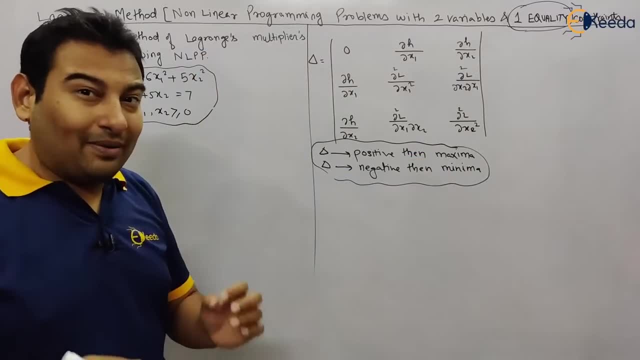 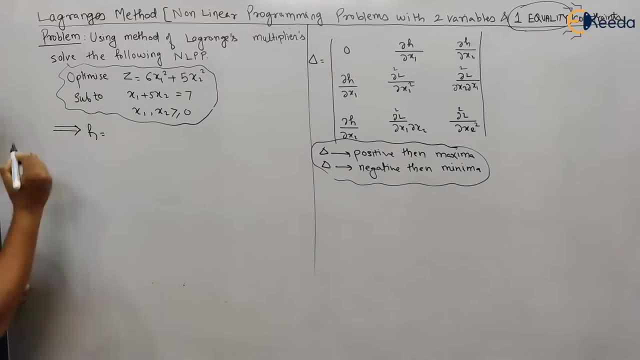 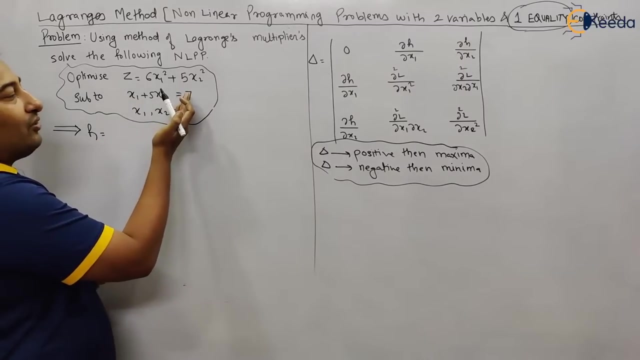 remember the condition based on that you're going to conclude. now you might be thinking: what is this h and what is this l that we're going to see here? so let us start. h means basically your constraint. see, this is your h and this h is basically: you take the 7 this side, so that is x1 plus 5, x2, 7 will. 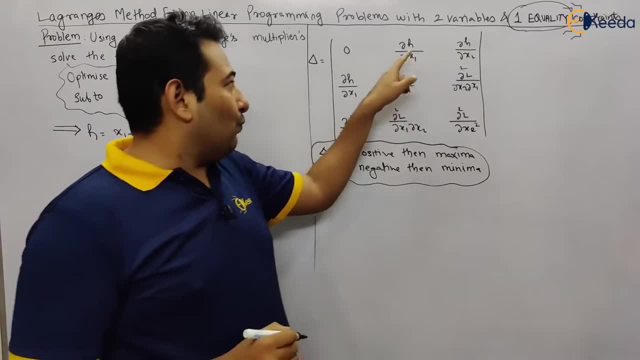 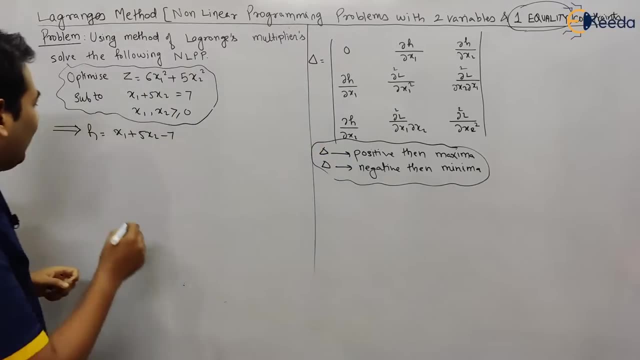 come to this side and will become minus 7. this is your h. we are ready with h. what else we want? we want l. l is your lagrange's multiplier and how to find l. l will be a function of x1, x2 and lambda. how come x1, x2 is given in the problem and there is one more variable that is lambda? 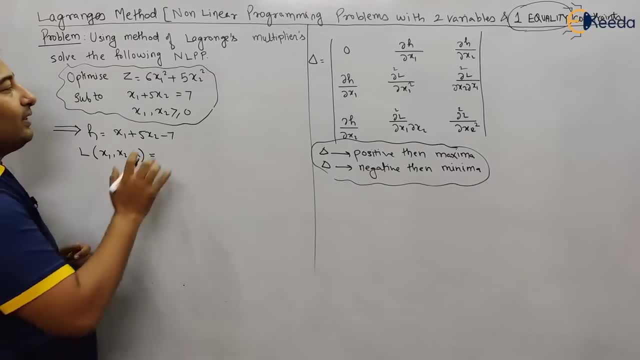 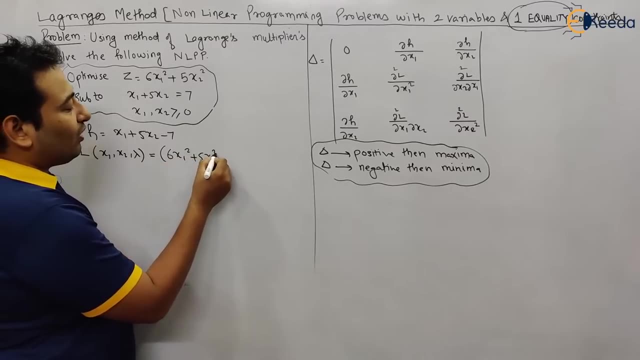 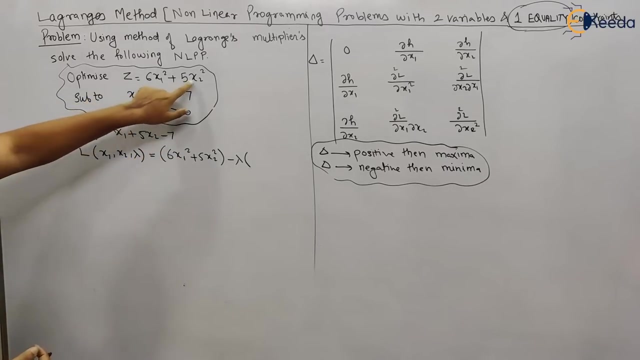 and how to write it down. lc, the method. first of all, we're going to write it down this: 6 x1 square plus 5 x2 square, minus lambda times constraint. first of all, write it down: the objective function. this is your objective function, this is your constraint. so, first of all, the 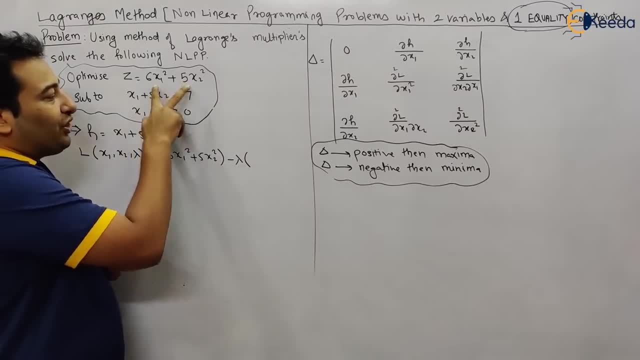 procedure is very simple, so we are going to write it down. this is your objective function. this is very fixed. the first of all, you need to write it down: the objective function minus lambda times, your constraint. and what is the constraint? this is your constraint, or you, this is your constraint. 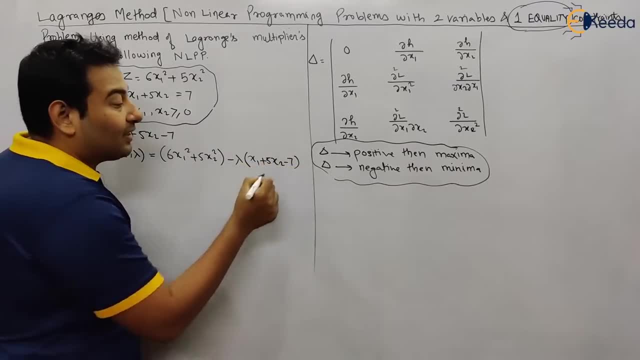 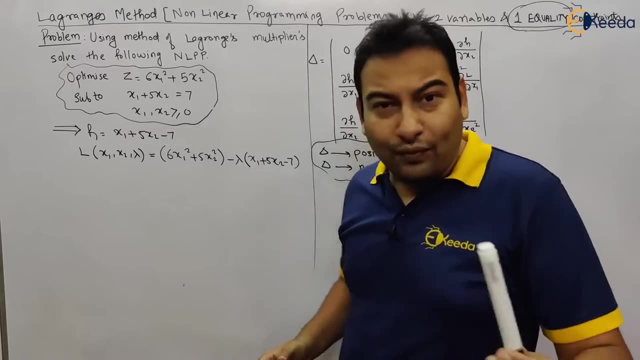 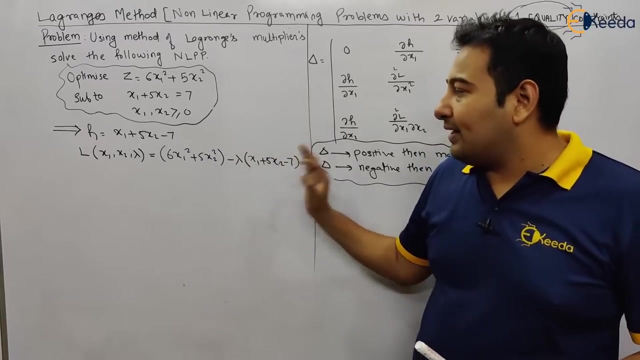 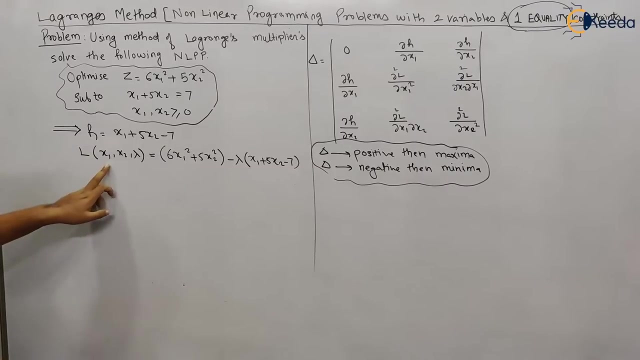 i hope this is clear. how to find l and l procedure is fixed. in the next videos also, we'll be discussing the same method for finding l. so how to find l objective function minus lambda times constraint, this is the way we gonna find it out l. so let us check first of all this: l we can differentiate with respect to x1 or x2 or 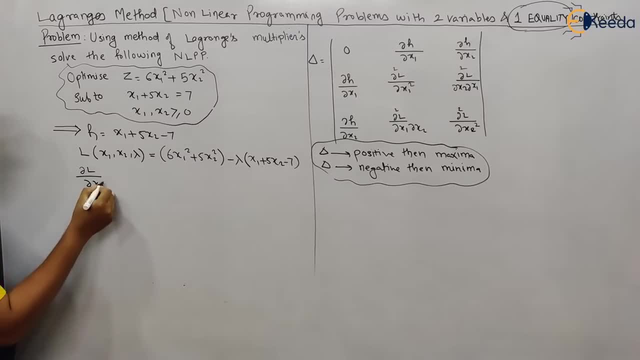 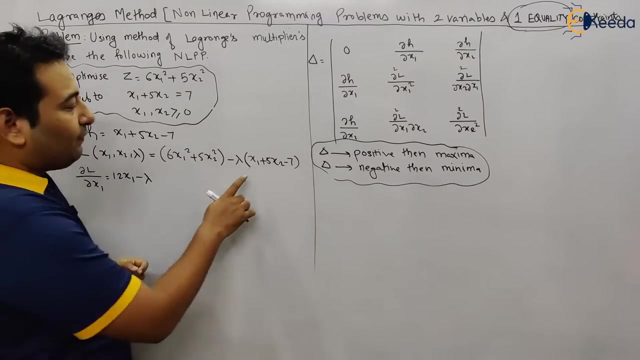 lambda. so let us do it. if you differentiate with respect to x1, so this will be 12 x1. i hope this is clear. 6 is constant, x1. square derivative is 2 x1. what about this minus lambda, if you differentiate with respect? see if you open this bracket. 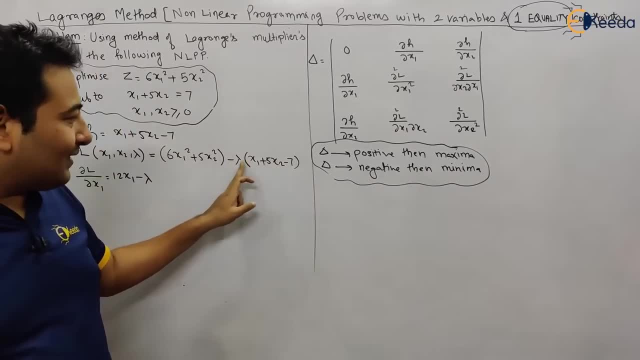 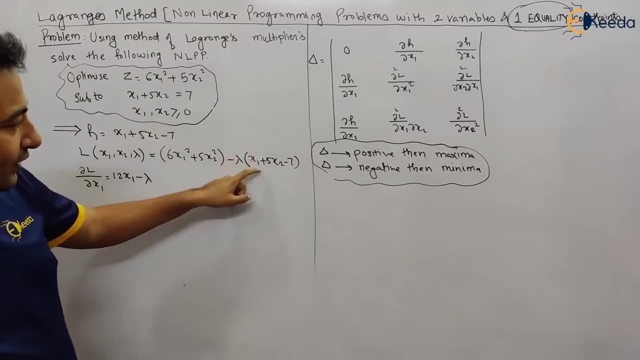 so please note that slash maxi is the fermion of x2 tilde. but what we've learned is here of if you have a number, can you do this. if you have a them, this is what you will be gonna be do all right. so now, when you do this, you will want to make sure that, if everything, 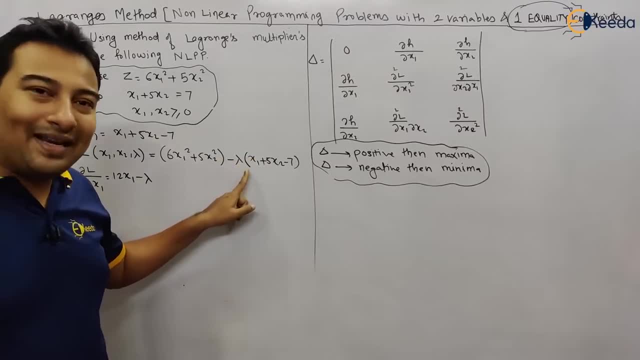 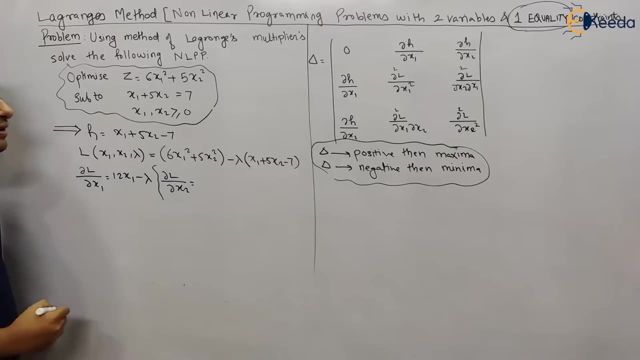 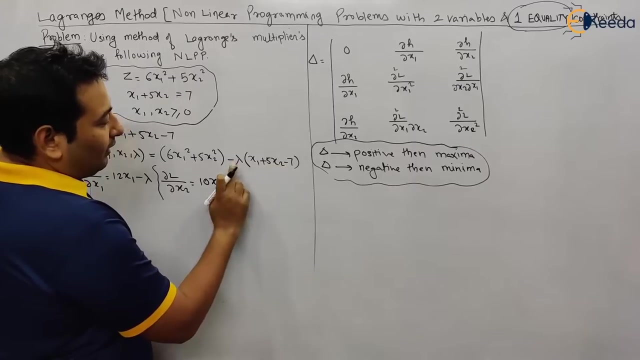 except the components x1 and x2 is constant and will take something as is at x1. this will have to be taken as a Town term, this single line on x mountain. so so what we need? solve this equation out okay. so herebound, this is the UM. so adoption of lambda x1 derivative. 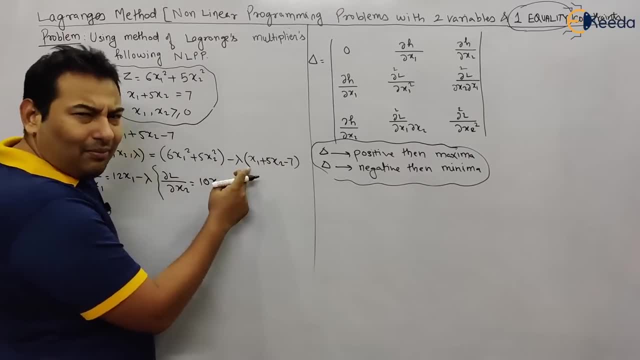 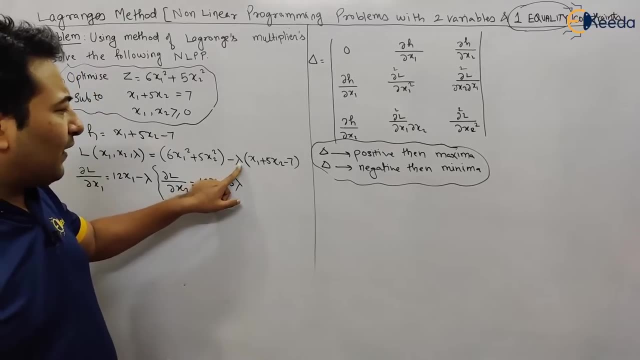 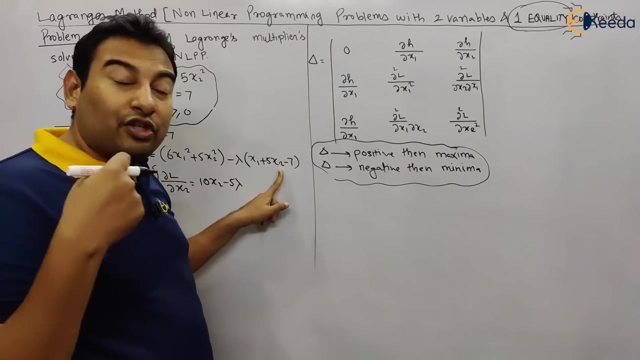 because we are differentiating with respect to x2. x1 is a constant term. lambda is also constant. we'll be left with this term, that is, minus 5 lambda. how come? very simple: minus 5 into lambda. if we multiply lambda inside, this will be minus 5 lambda x2. we are taking derivative with respect. 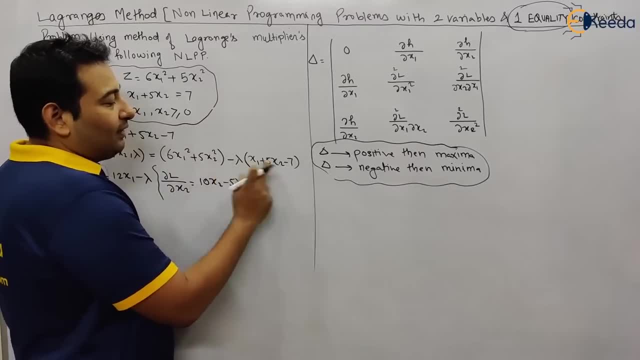 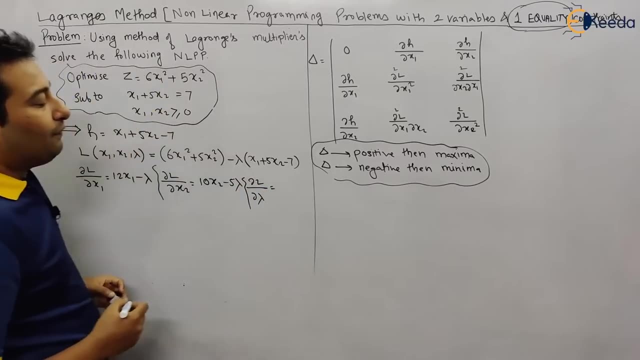 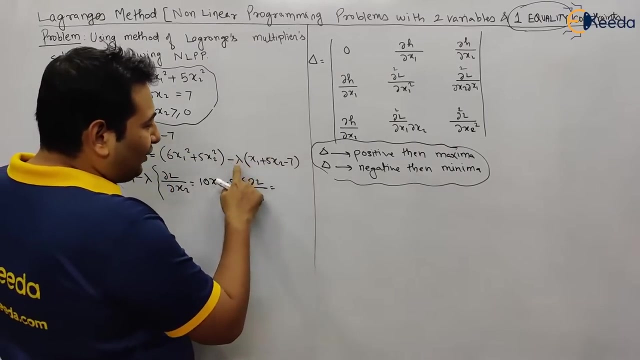 to x2, so that will be minus 5 lambda and obviously this term is a constant derivative: 0. what is last? now we're going to differentiate with respect to lambda. similar procedure with respect to lambda. obviously this will be 0. and if you differentiate this, 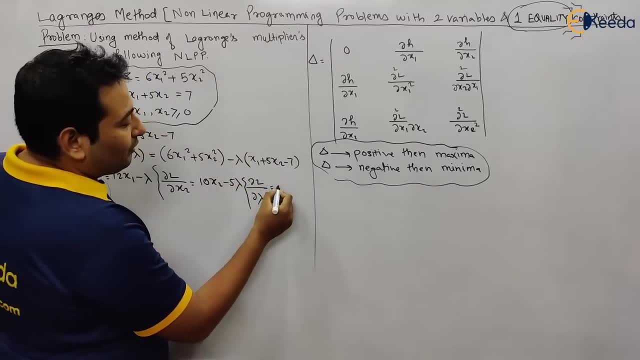 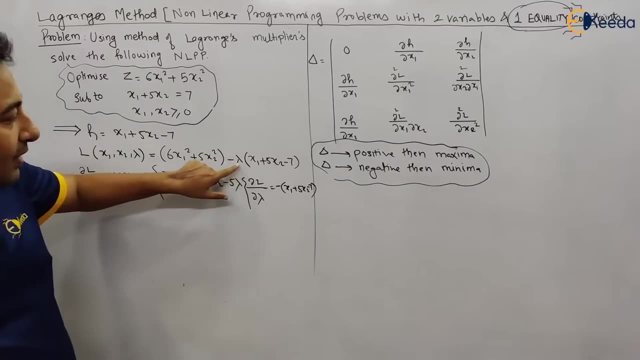 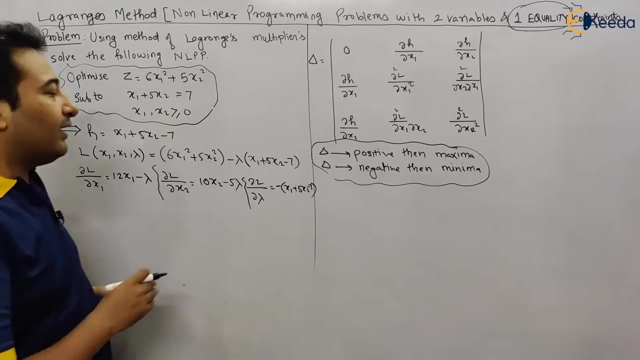 equation. with respect to lambda, this is a constant, so minus x1 plus 5x2 minus 7, see it with respect to lambda. if you're differentiating x1- x2 constant, its derivative is 0. with respect to lambda, This will come along with minus sign because lambda derivative is 1.. 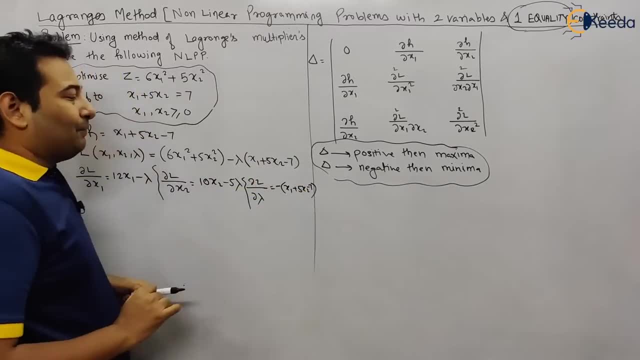 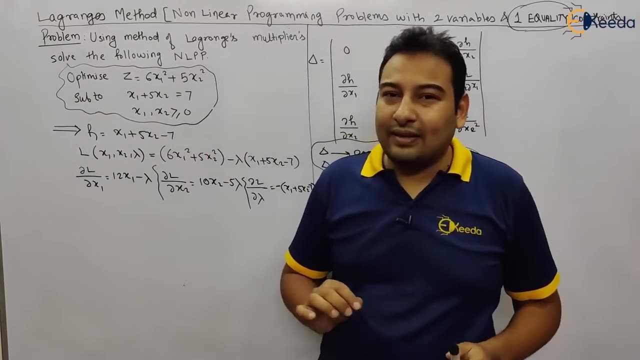 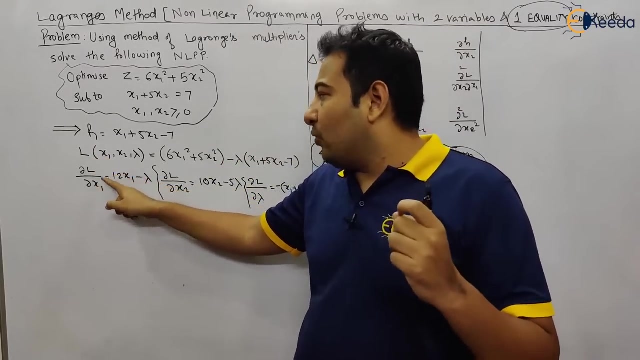 So lambda derivative is 1.. So this will come along with the minus sign. Remember type number 1, the previous type, in which also we did the same thing. There we wrote f of x1, x2, x3 and we differentiate f with respect to x1, x2 and x3. 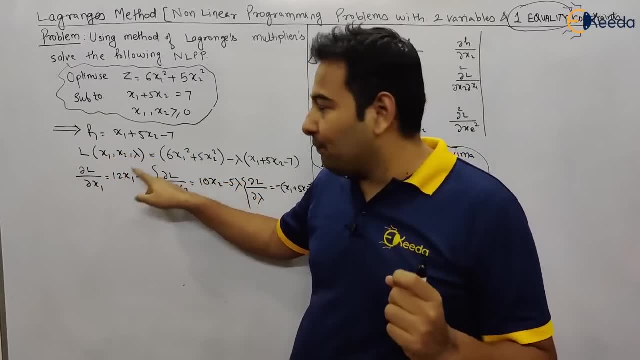 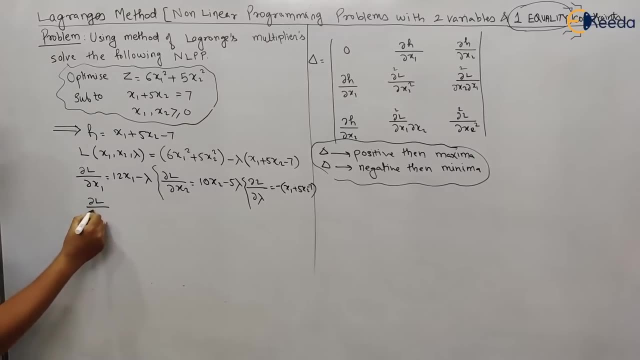 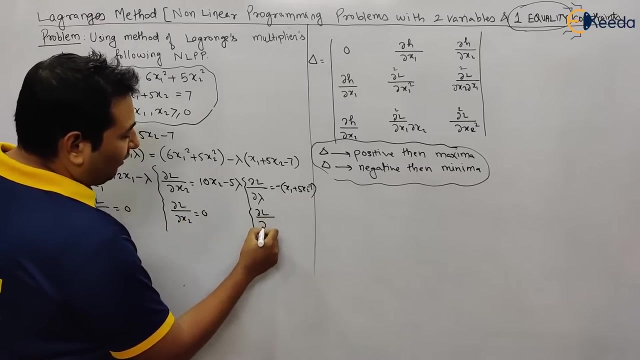 Here this L is a function of x1, x2, x lambda. Therefore, we need to differentiate with respect to x1, x2 and lambda. What next Similar procedure: We are going to equate it to 0.. This particular chapter, throughout the chapter. this is actually procedure oriented chapter. 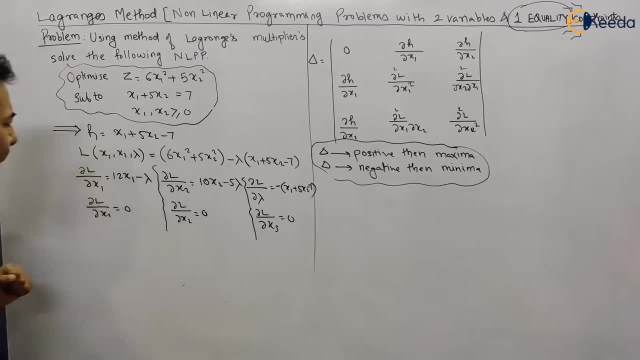 So you need to remember the steps and you need to follow the steps. You will get your result With respect to x1, 0. So this will be 12x1 minus lambda, equal to 0.. Then x2 minus 5 lambda, equal to 0. 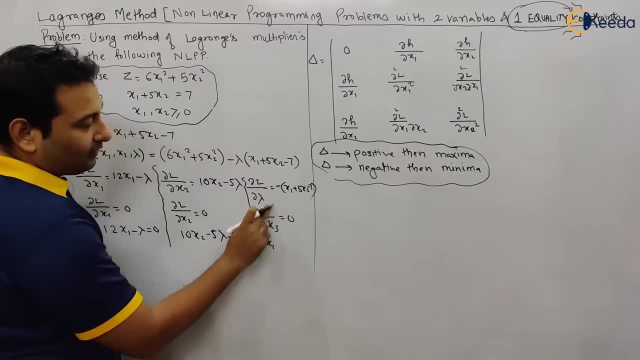 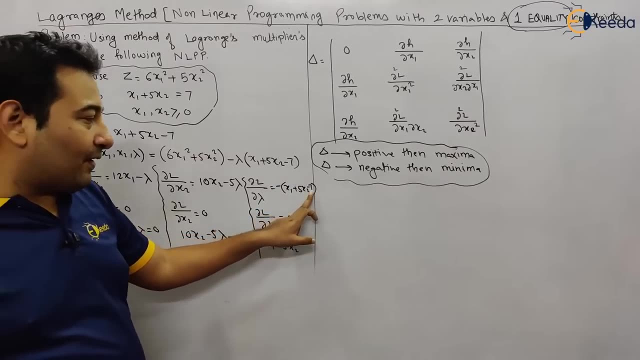 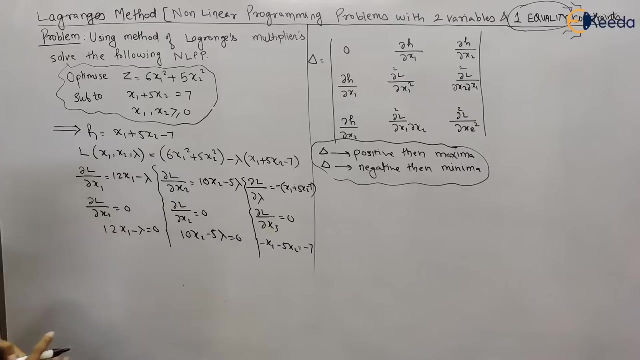 And if you open the brackets, this is minus x1.. See here, This is minus 5x2.. And this is plus 7.. But plus 7 will go to that side and will become minus 7.. Minus x1, minus 5x2, plus 7.. 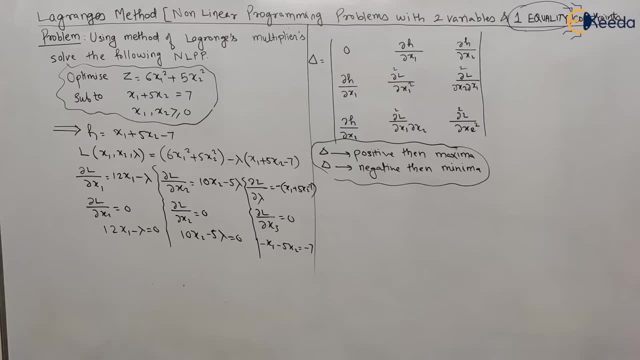 Plus 7 will go to that side of equal to and that will become minus 7.. Now you are ready with 3.. You need to solve these 3 equations in calculator to get the value. After solving you will get: x1 is equal to 7 upon 31.. 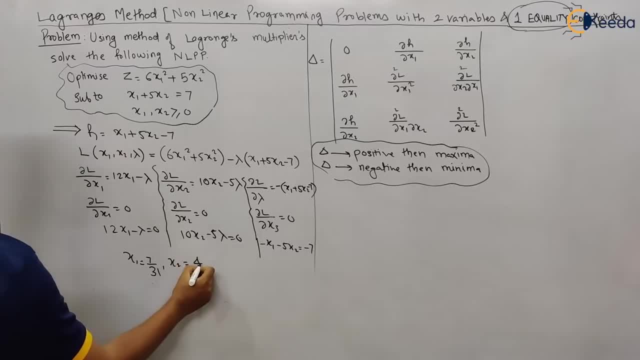 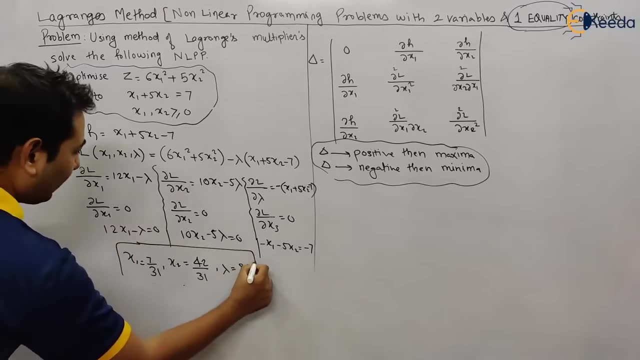 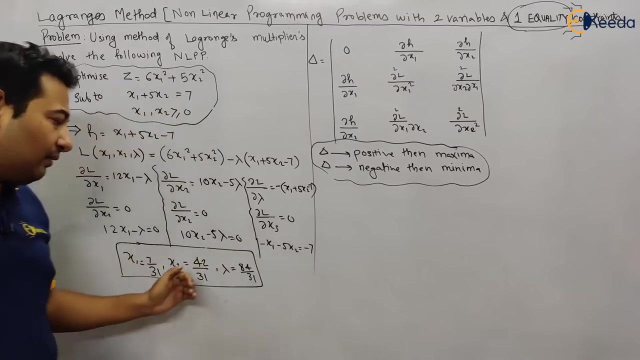 x2 is equal to 42 upon 31.. And lambda is equal to 84 upon 31.. You can check your result in calculator. You will get it. It's very simple. Solve these 3 equations in calculator In a proper way. you will get your result. 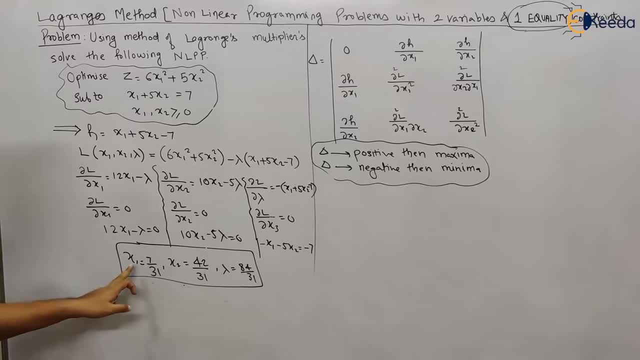 So x1, x2, we are ready with lambda. If we put x1 and x2 in this particular equation, we will get the value of z. The only thing left is we need to check whether the answer that we are getting is a maximum value or a minimum value. 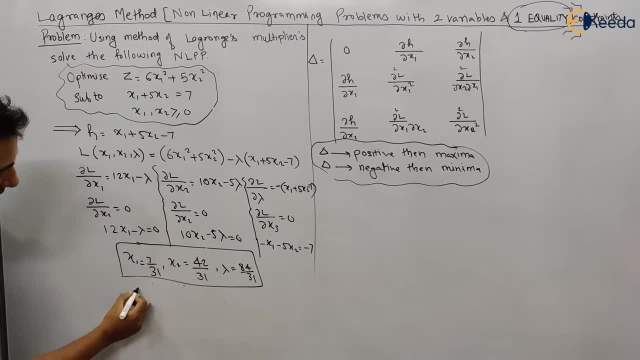 So let us put x1, x2 in z. If we put, we will get 294 upon 31.. You can check. The only thing left What I am doing: x1, x2, I am subtracting. 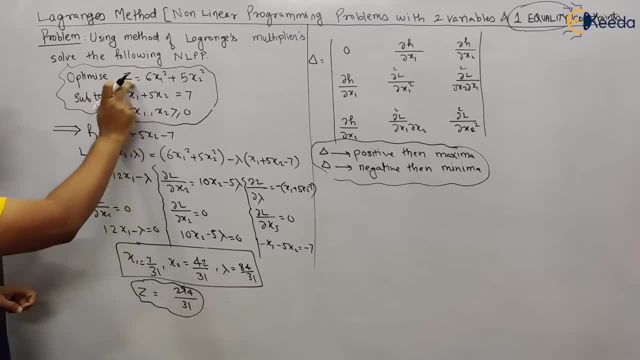 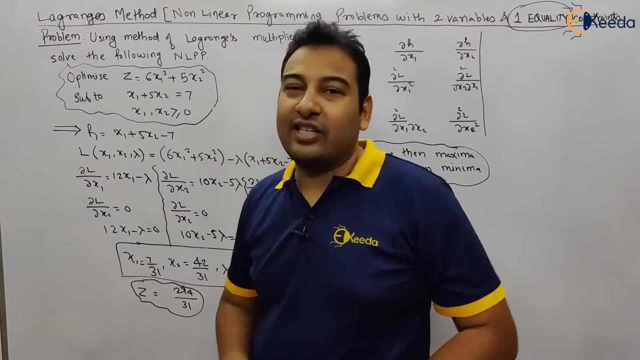 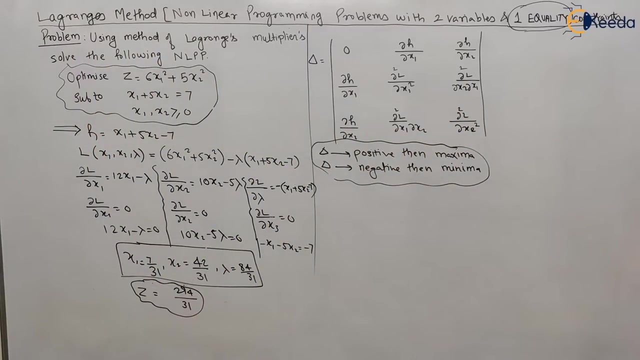 Here, x1 and x2 put here and get the value of z, and z value is coming out to be 294 upon 31.. The only thing left here is to write it down, whether it is a maximum or minimum, and who will decide that? this delta will decide whether the term is a maximum term or minimum term. 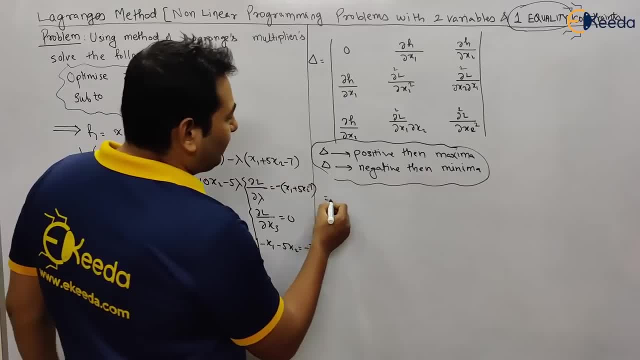 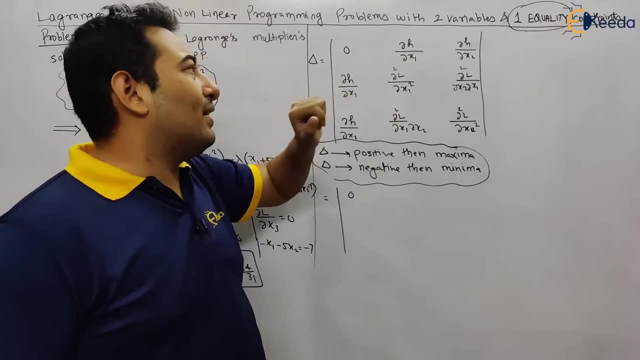 So let us quickly find it out, the things that will be required for this particular matrix. See, here it is dou h upon dou x1.. That means we are going to differentiate h with respect to x1.. So where is h? 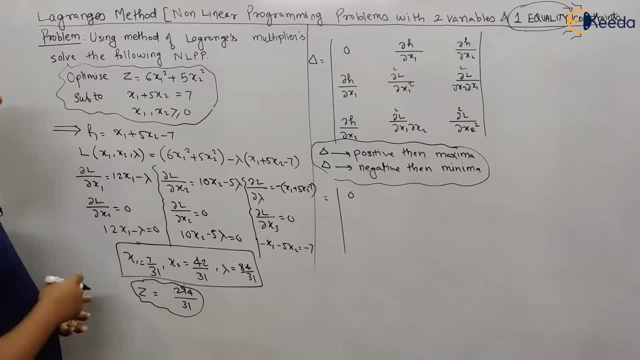 See here, let us differentiate with respect to x1.. So, with respect to, if you differentiate with respect to x1, so this is 1, both the terms are constant. its derivative is 0, only 1.. With respect to x2, this is 0, this is 0. 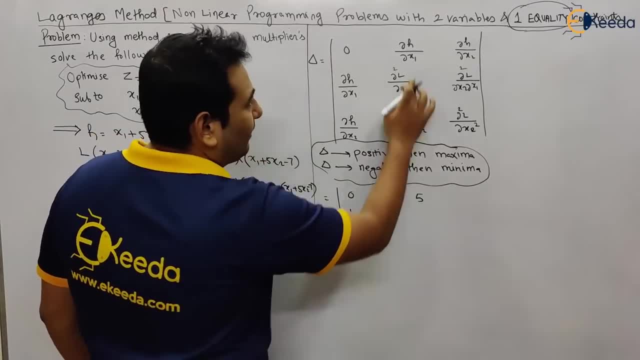 With respect to x2, we will get 5.. Again, this is 1 and 5 because the terms are same: dou square l upon dou x1 square. That means we are going to differentiate h with respect to x1.. 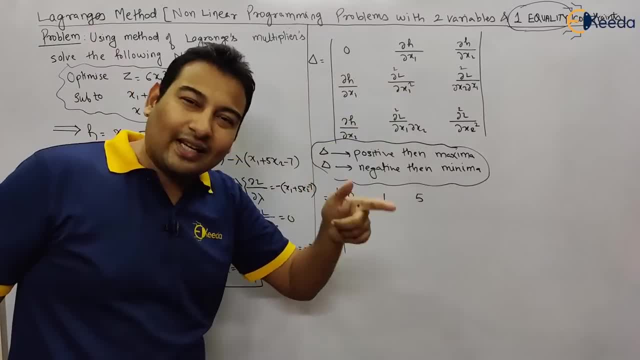 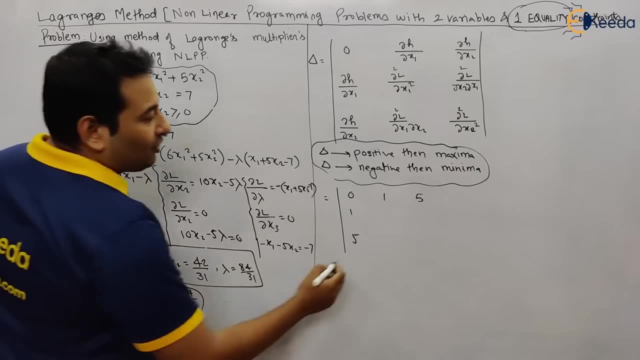 Since dou l upon dou x1, we already got it- we are going to differentiate once again with respect to x1 partially. So the answer will be 12. because this is constant, its derivative will be 0. So here it will be 12.. 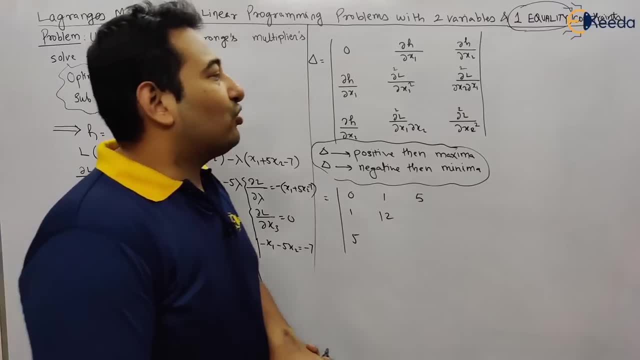 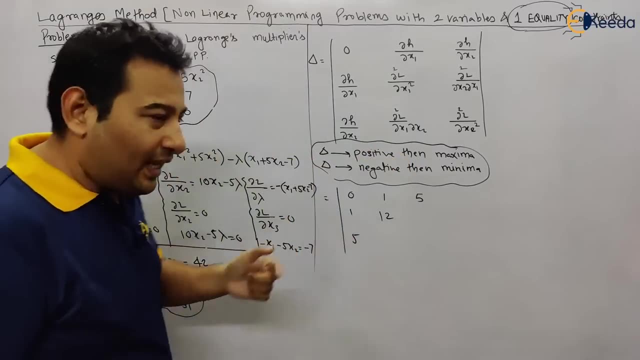 Next, dou square l upon dou x2, dou x1.. It is very simple. You differentiate dou l upon dou x1 with x2 or dou l upon dou x2 with x1.. One and the same thing, So this is dou l upon dou x1.. 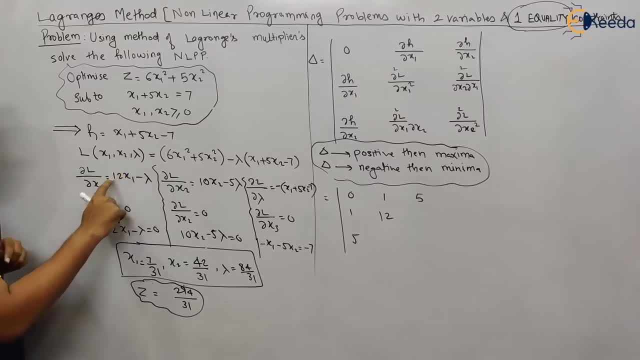 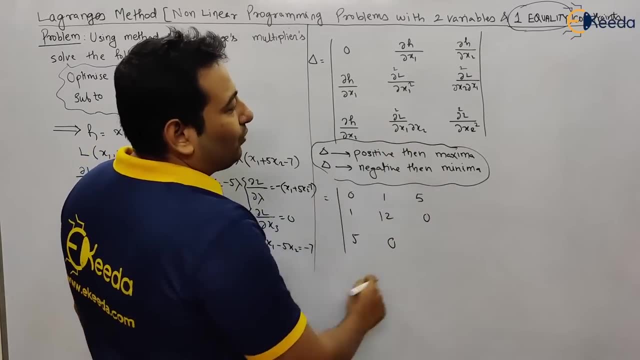 Let us differentiate with respect to x2.. With respect to x2.. The entire term is a constant. Its value will be 0.. What next? Again, this is 0.. With respect to x2, if you differentiate, that is 10.. 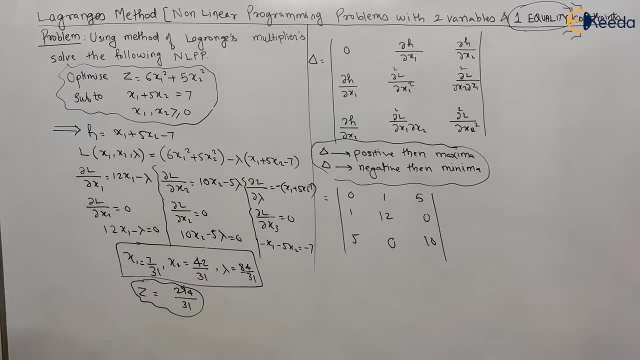 Now we need to find it out, this determinant, to check whether the answer that we are going to get is a maximum or minimum. So this determinant, you can directly put it in calculator Or you can solve manually also, There is no problem. 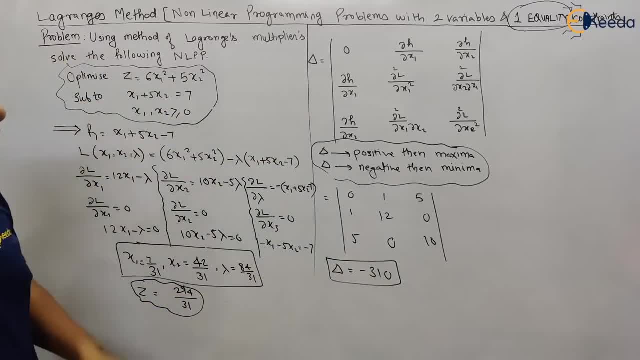 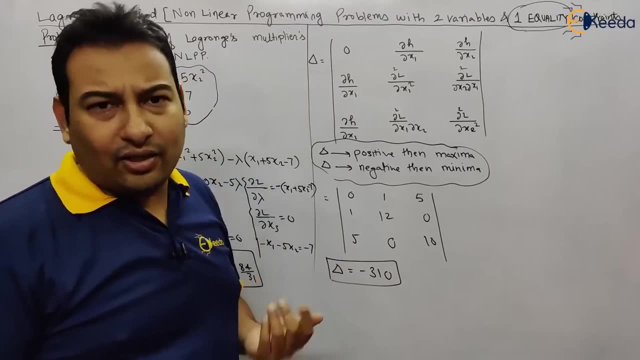 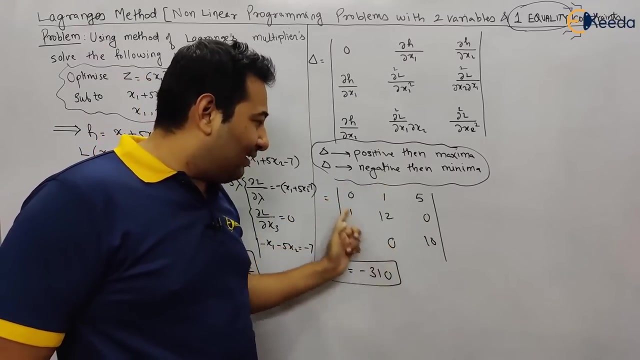 You can directly put this determinant in calculator, because calc is allowed in the exam. So you can put in calculator, or you can directly get the answer, or you can solve manually. This second term will be minus. Leave this column, this row and so on. 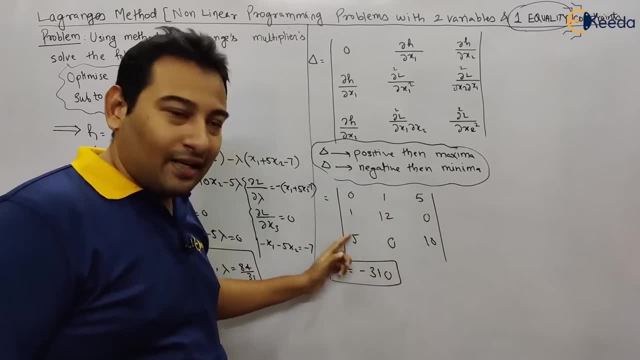 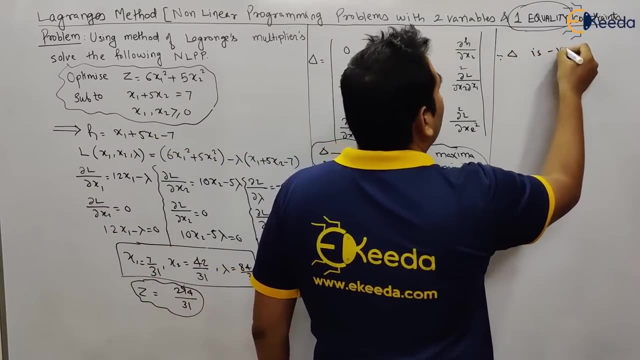 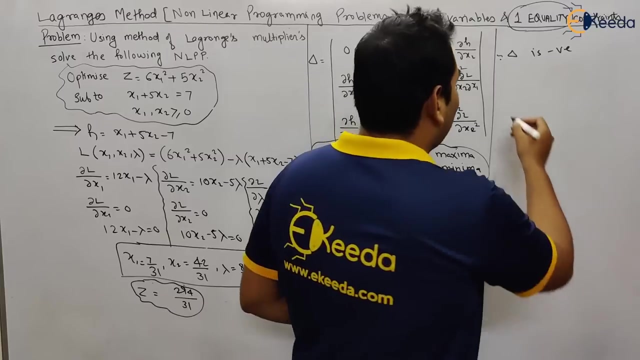 This is the procedure. I hope you know this procedure. So delta is negative. See here: Delta negative. What does this indicate? Since delta is negative, that means the answer that we got z value. If delta is negative, then it is a minima. 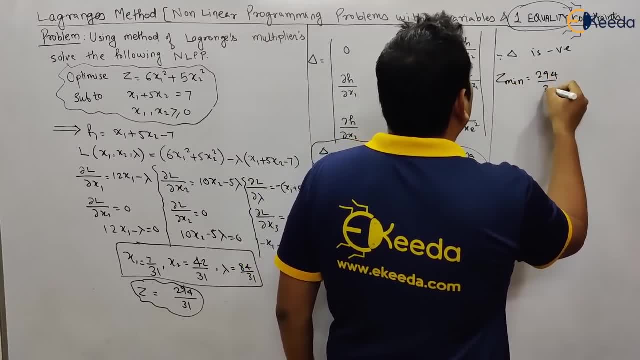 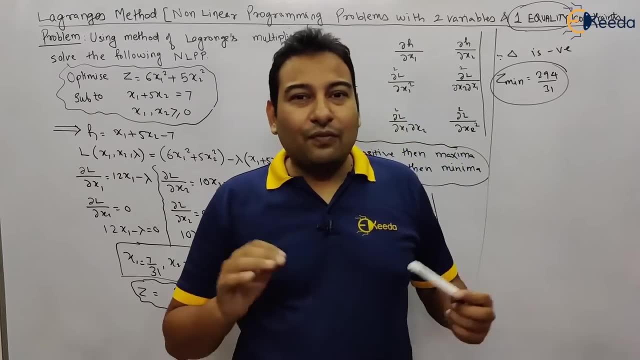 So z mean is equal to 294 upon 31.. So this is your required solution for this particular problem. This problem is exactly similar to the previous problem, in which there was no constraint, So only difference is there is a constraint involved. 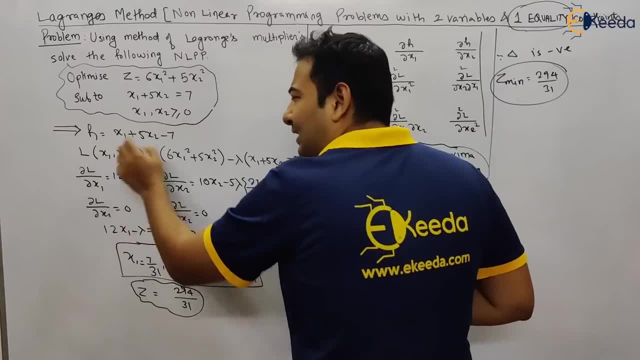 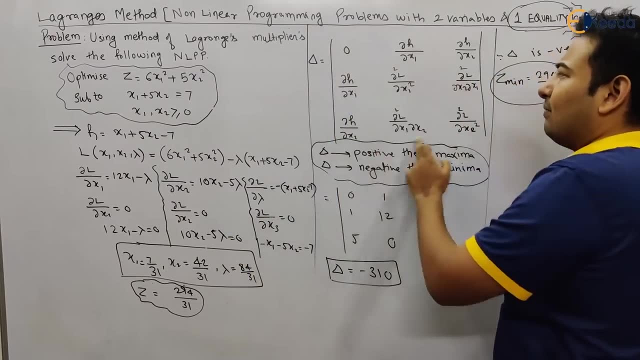 So first of all you need to find it out L and this procedure is same: X1, X2, lambda differentiate- There it was a hashen matrix, Here it's a delta to determine whether it is a maxima or minima. 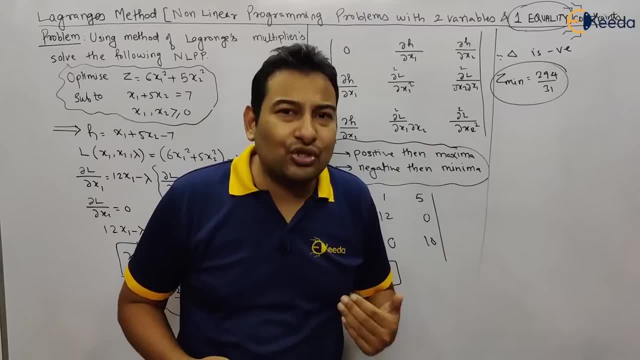 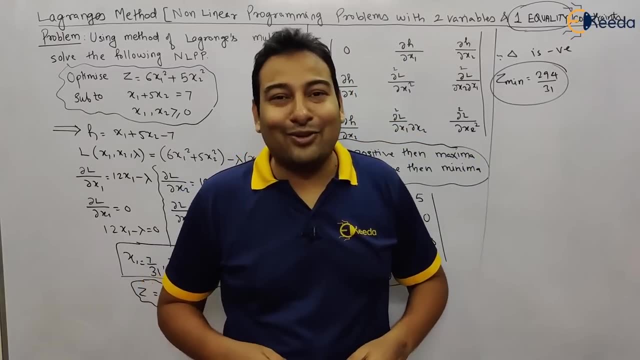 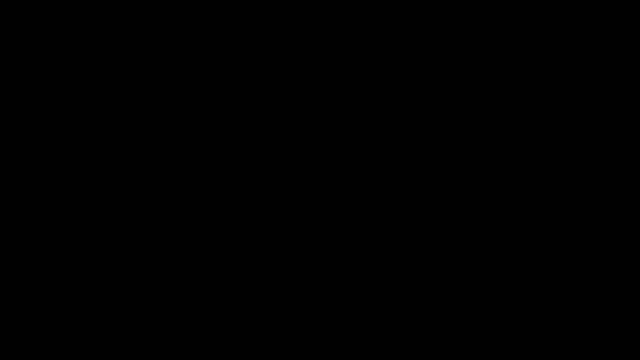 So go through this video once, twice and understand the procedure, because remaining problems are also same. All the problems of the same category are same. Hope you understood. We're done with it, Thank you. Subtitles by the Amaraorg community.